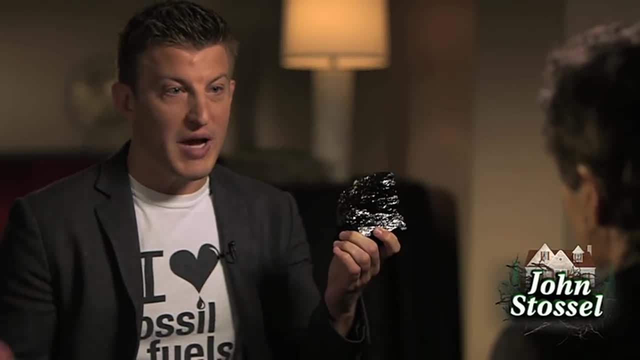 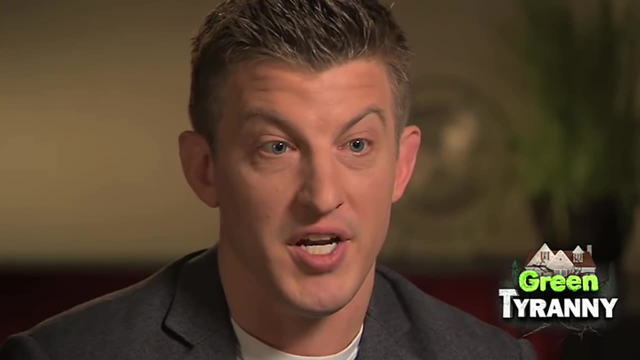 and figuring out how to use it to charge your iPhone or to power your car. I think that's amazing. It is amazing, but it pollutes. Energy is a climate protection device and we need as much of it as we can get. 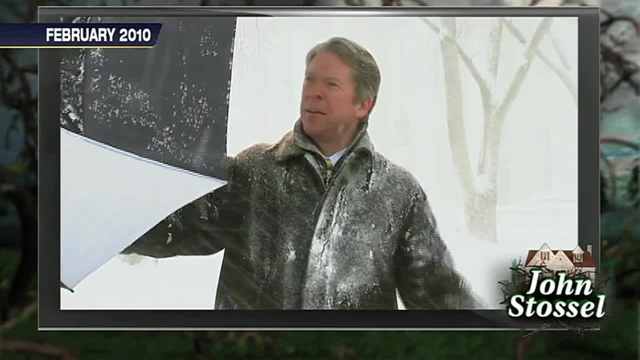 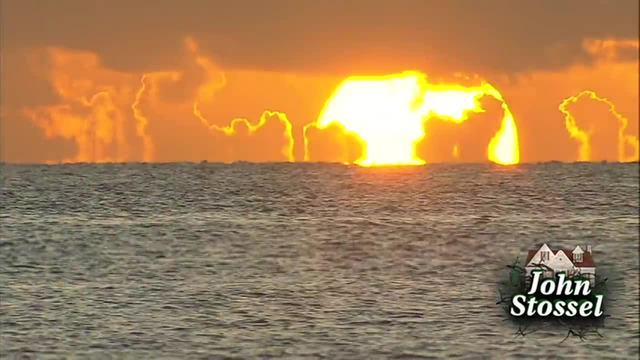 There we go. This is what we do on live television, folks in the blizzard. Nature doesn't give us a safe climate that we're making dangerous. It gives us an incredibly dangerous climate that we're making safe- Certainly safer, Even as the globe has warmed. 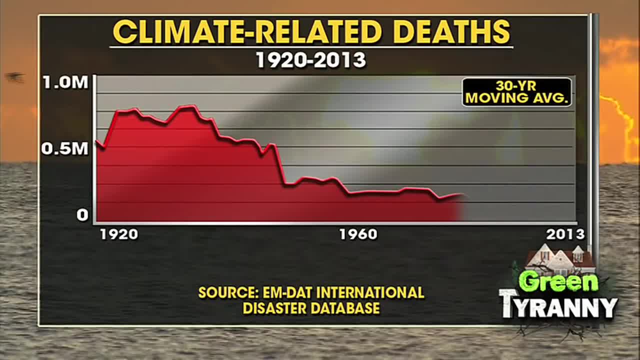 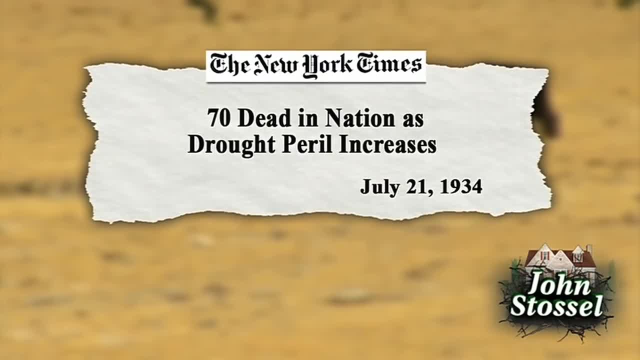 climate-related deaths have dropped by a lot Since 1933, by 98%. We desperately need the rain. Drought used to be the biggest climate-related killer, but those deaths are way down because fossil fuels allow trucks to bring food to people. 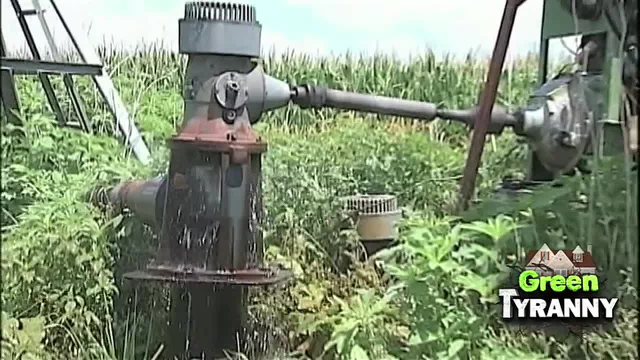 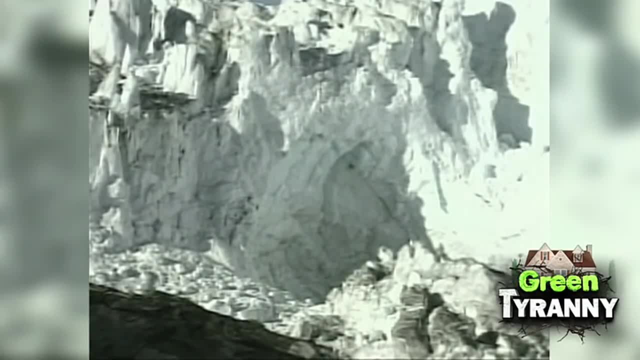 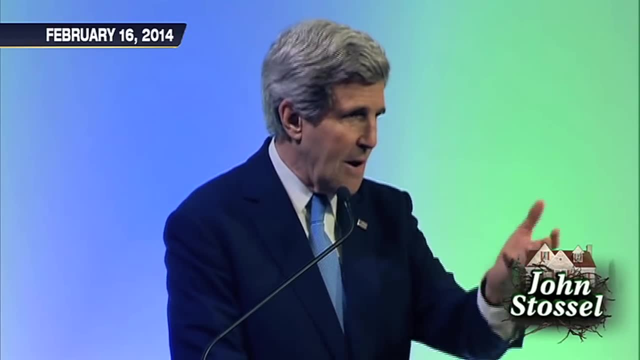 who once starved, and because farmers fight drought with fossil-fuel-powered irrigation pumps. Still, global warming may become a big problem. All the worst predictions. If they never materialize, what will be the harm that is done from having made the decision to respond to it? 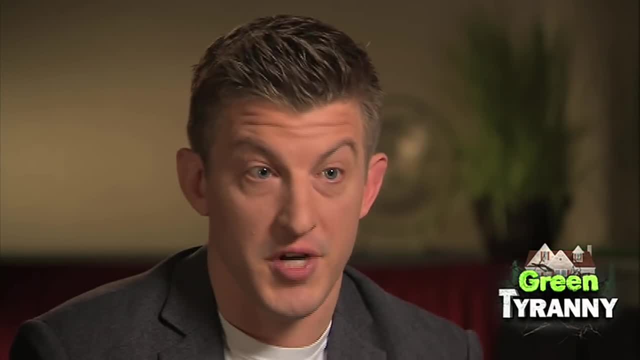 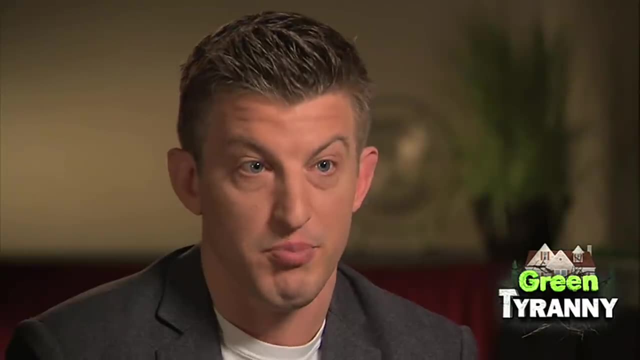 What's the harm? Kerry was giving that speech in Indonesia. If they hadn't been able to use coal, which is what Kerry thinks they shouldn't be able to use- they would still be desperately poor, But the protesters don't think about that. 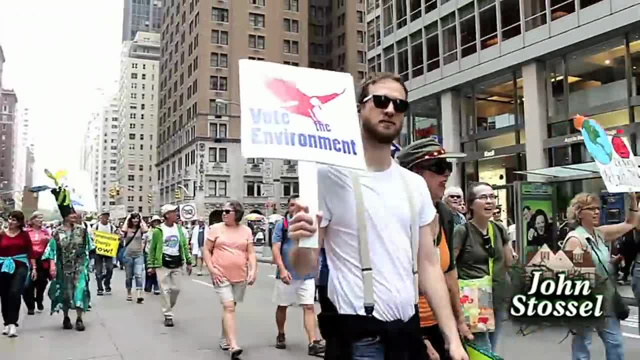 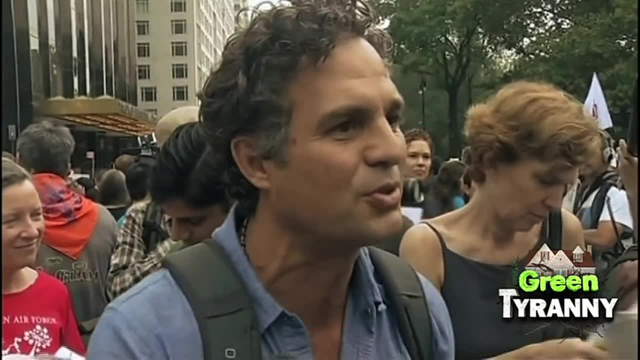 And the green tyrants have convinced them. other fuels are just as good. Renewables really work. 100% renewable for Americans means Americans get to control and own their own energy. Politicians, give your money to people who sell wind power and solar power. 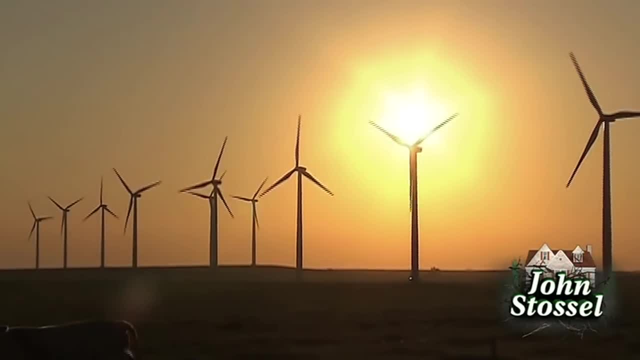 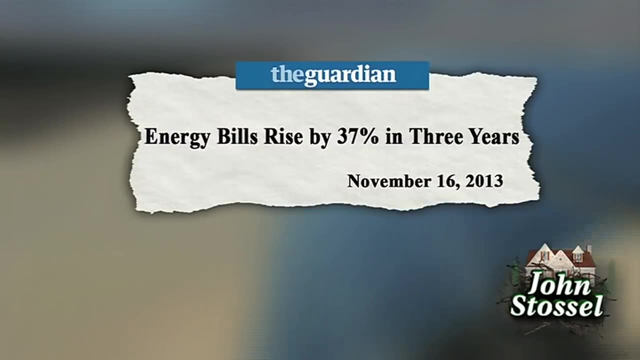 We've got to keep developing new sources of energy. Europe tried that first, but then noticed the wind doesn't always blow And clouds sometimes block the sun. Electricity prices shot way up, So now in Europe Many governments are reinvesting in fossil fuels. They're actually building more coal capacity than ever to compensate for the renewables that they can't rely upon. Sometimes there's too much, sometimes there's too little. You want forms of energy that you can control, not that control you. But activists point out, renewables are improving. 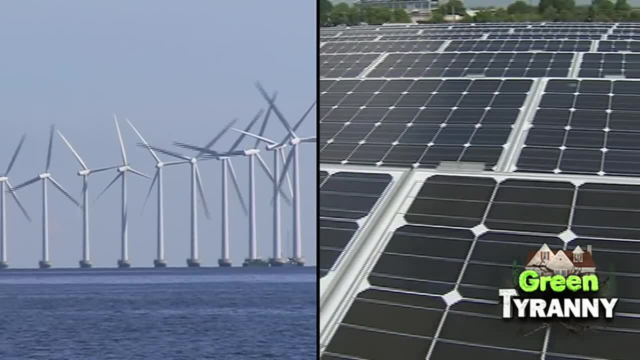 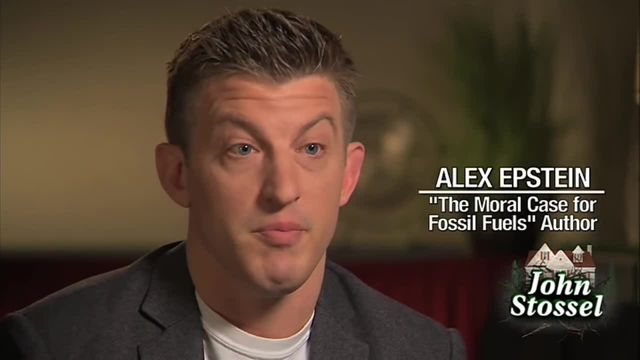 Today they provide 13% of America's electricity. However, When people say renewable, they usually think solar and wind, But those contribute a very minuscule percentage. It's mostly hydro, which is a great source of energy that the environmentalists mostly oppose.